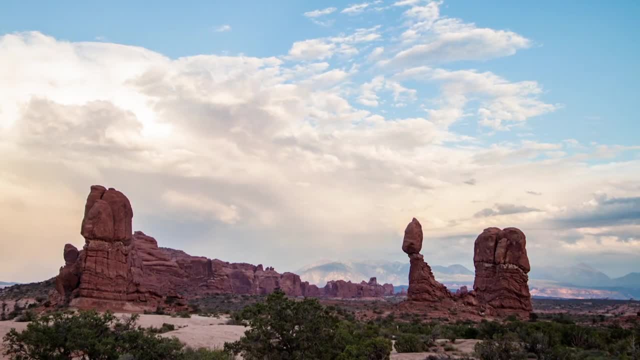 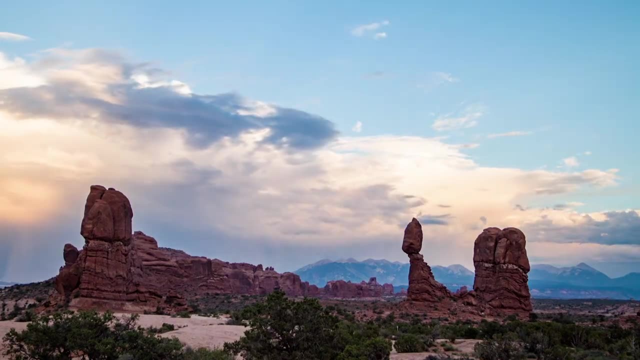 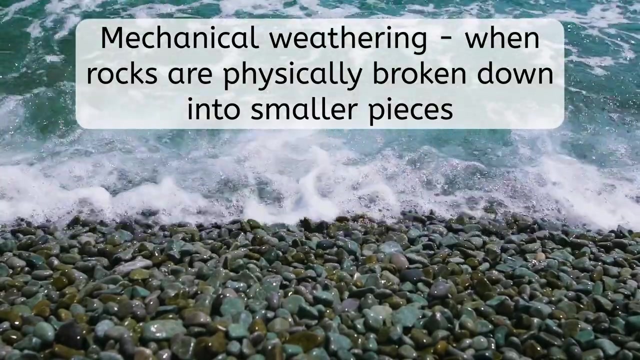 effects on our planet. One of these slow processes is called weathering. There are two different kinds of weathering: Mechanical weathering and mechanical weathering. Mechanical weathering and mechanical weathering is when rocks are physically broken down into smaller pieces. There are tons of 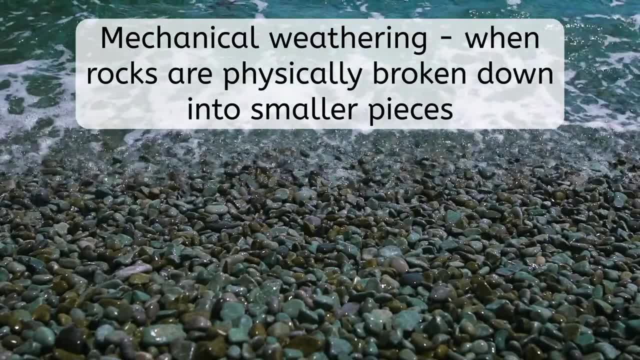 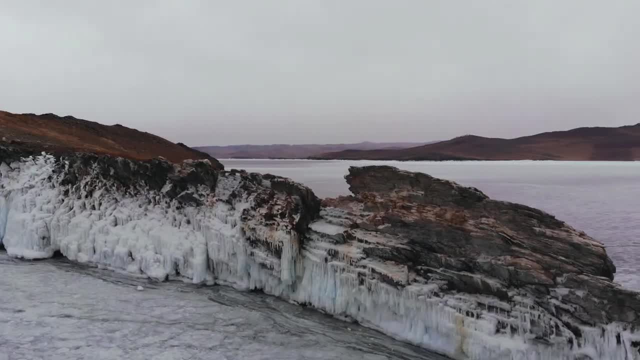 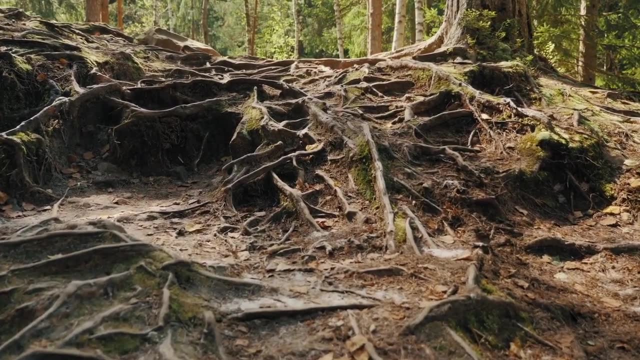 different ways this can happen. The constant pressure from wind or moving water can chip away at rocks. over time, Water can also get into cracks in the rock, then expand and push outwards when it freezes. Even plant roots can cause mechanical weathering by breaking stones apart. The important 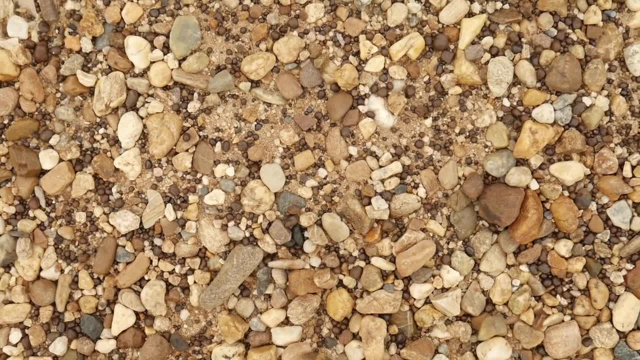 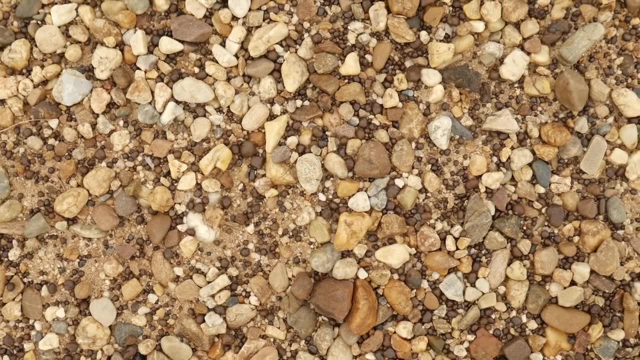 thing to remember about mechanical weathering is that while it breaks the rock apart, it doesn't change what the rock is made of. It basically just creates tiny pebbles and sediments of the same composition. Think of it like the world hitting a rock with a hammer- except the hammer. 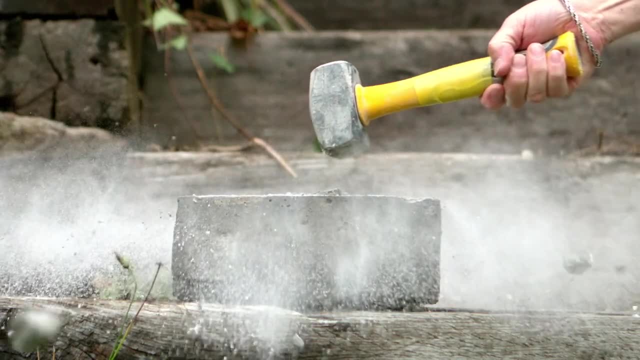 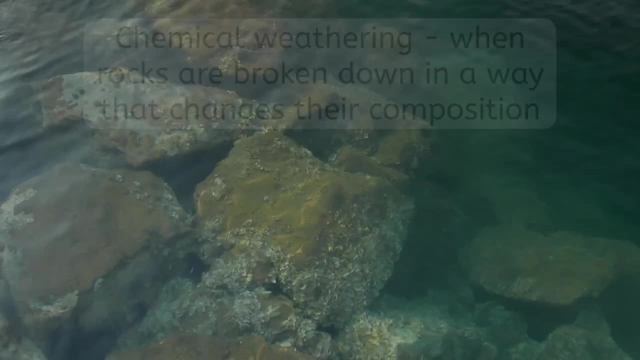 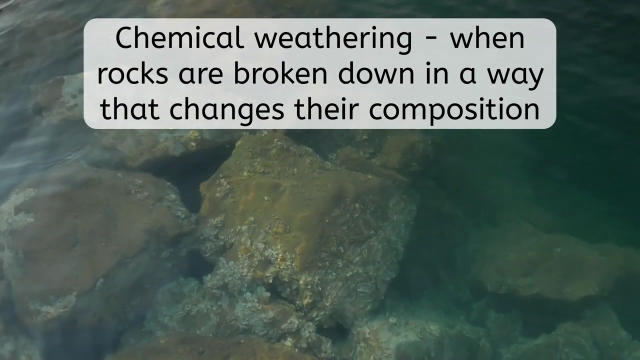 is something like the wind or a river. Alright, I admit it's not a perfect metaphor, but you get it. So that's mechanical weathering. On the other hand, chemical weathering can change a rock entirely. This is when rocks aren't just broken down, but their composition is also changed. Ever seen a 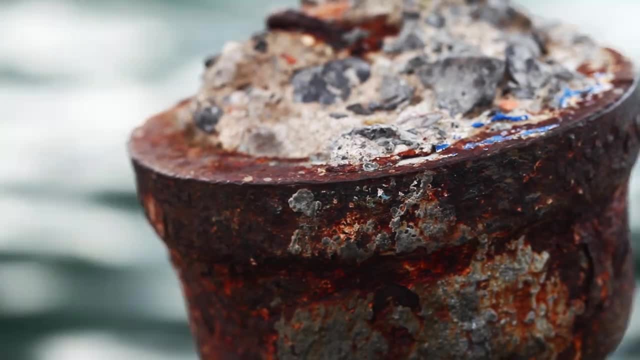 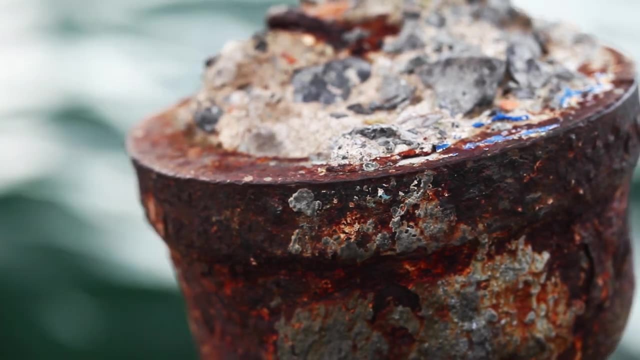 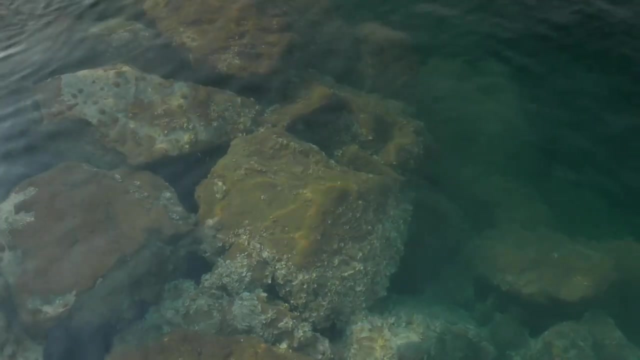 piece of metal get rusty after it sits outside. That's an example of chemical weathering. The oxygen in the air actually caused the metal to undergo a chemical reaction which changed its entire composition and broke it down in the process. Chemical weathering also occurs when 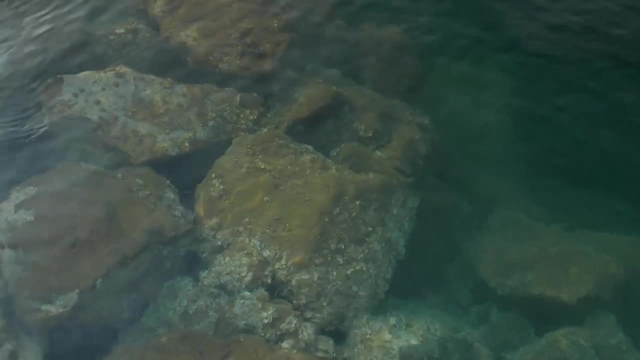 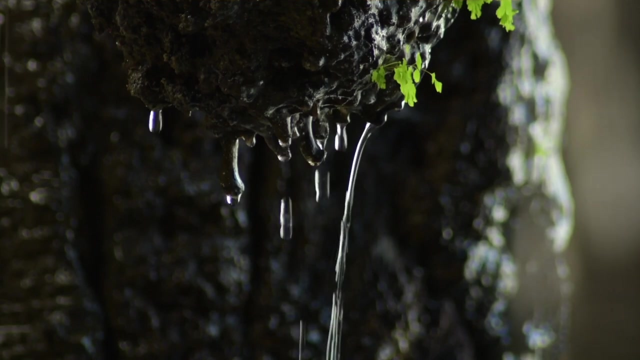 rocks react with something like oxygen or water. Stalactites in caves can cause the rocks to break down, but they can also cause the rocks to break down. These rocks are formed when minerals in cave rocks dissolve into water. Then the water drips down and leaves the buildup of minerals. 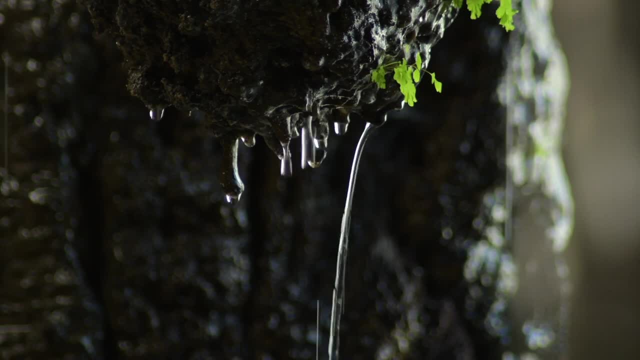 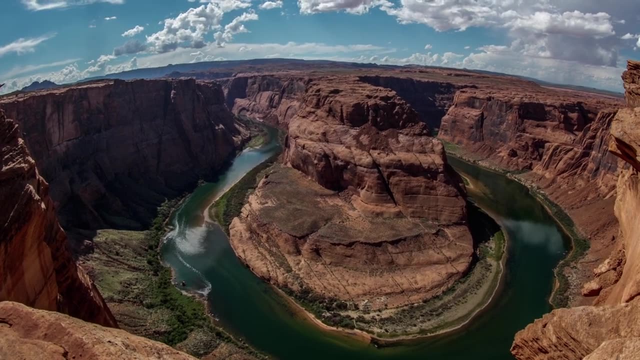 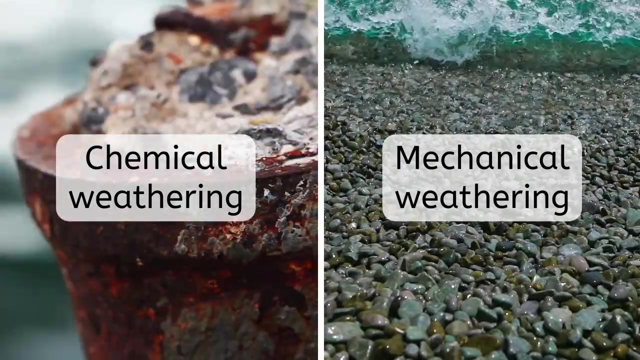 behind Chemical and mechanical weathering. both shape our planet in countless ways. Both chemical and mechanical weathering can involve some of the same forces, like air and water. The difference comes from how these forces break down rocks. Chemical weathering actually changes the structure of rocks. The rocks break down, but they don't break down Chemical weathering. 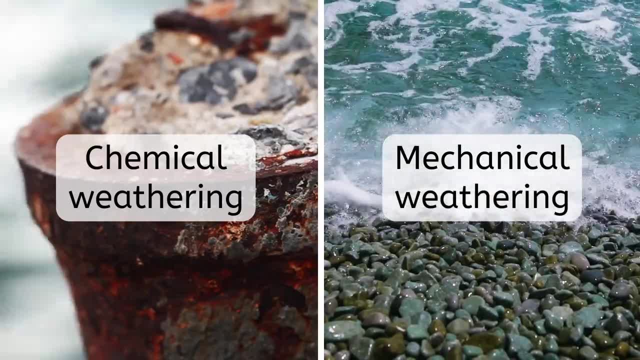 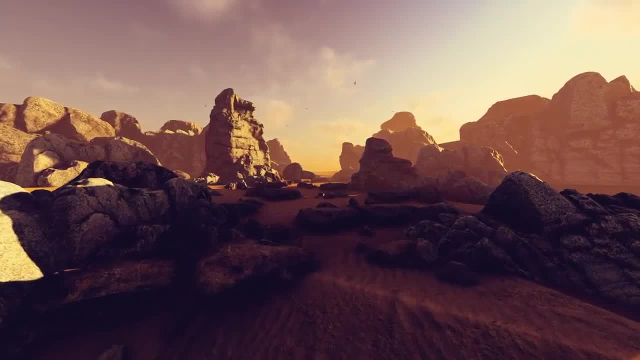 actually changes the structure of rocks. Chemical weathering actually changes the structure of rocks. This is what the rock is made of, while mechanical weathering mostly just crushes it up. A few different things can affect how fast these processes happen. too High temperatures result. 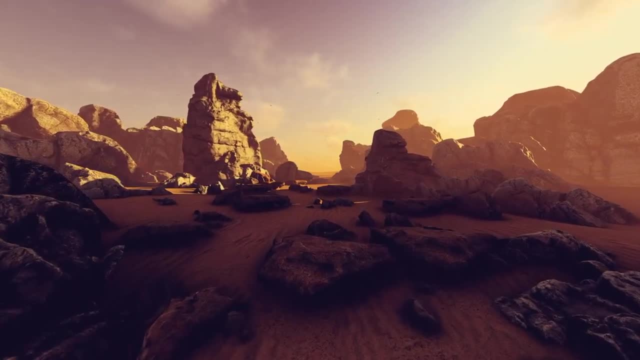 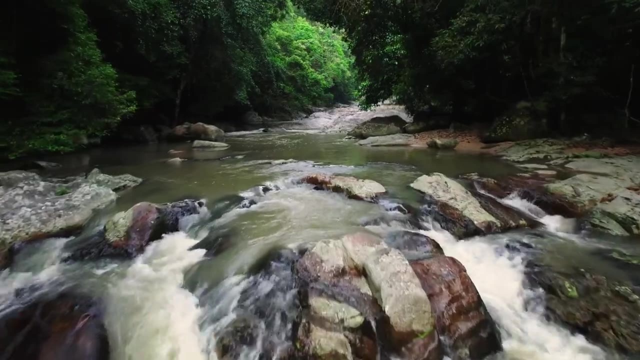 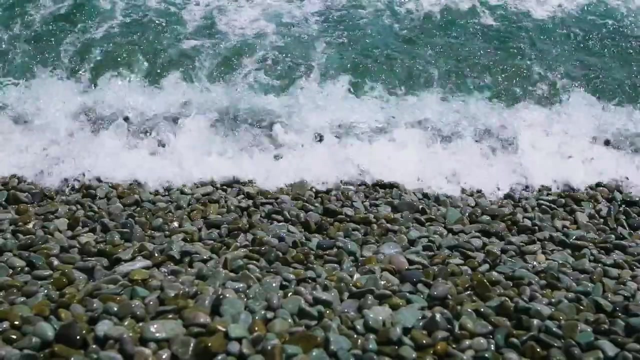 in rocks weathering faster than cold temperatures. Higher levels of rainfall and humidity do too. So rocks in the hot, rainy tropics weather much faster than rocks in the cold, dry Arctic. Now you might be wondering if these processes are. 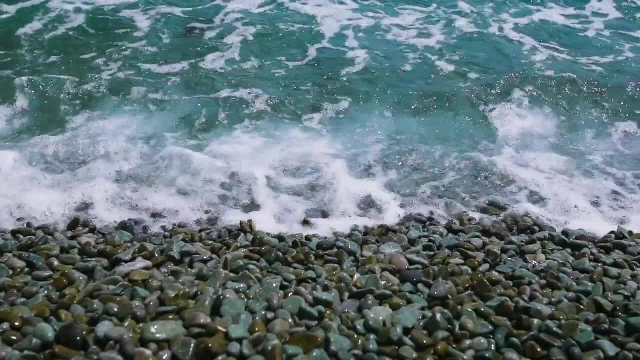 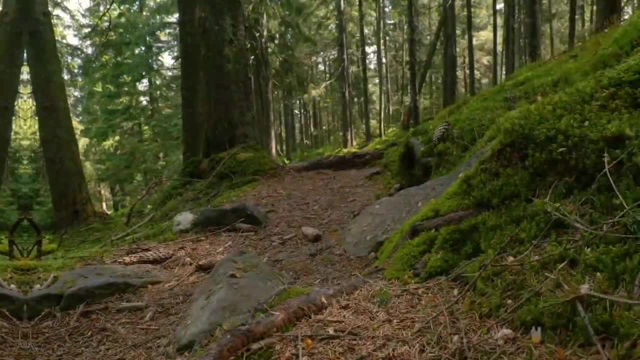 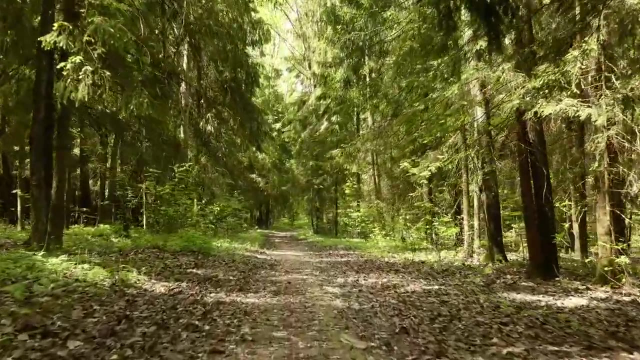 constantly occurring and breaking rock into tiny pieces. well, where do all those pebbles end up? And, although it might surprise you, the answer is here And everywhere, really. Every time you go for a hike outside, sit on the grass or even plant a garden, you're seeing what the next step is for. 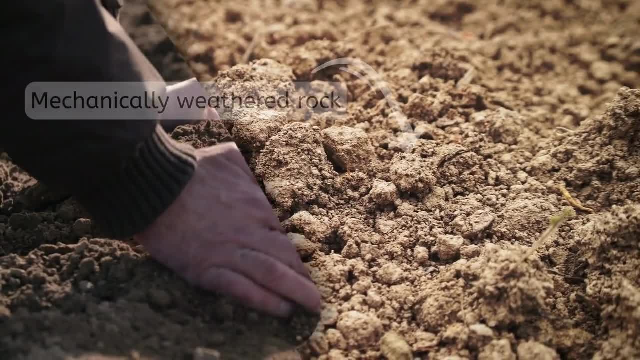 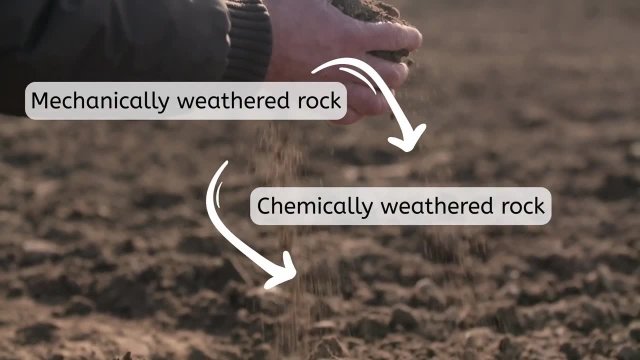 those weathered rocks Soil. Mechanical weathering breaks rocks down into fine pieces that make up part of the soil. Mechanical weathering breaks rocks down into fine pieces that make up part of the soil. Chemical weathering breaks them down into the minerals that enrich the soil. 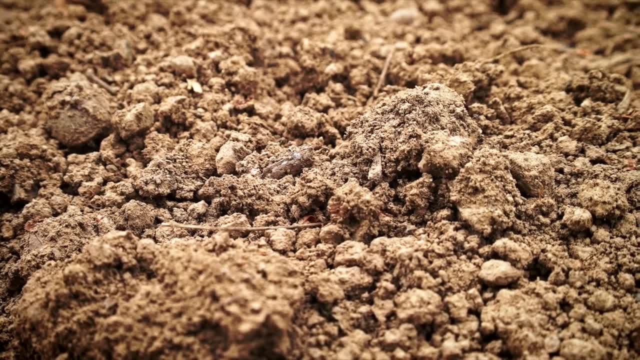 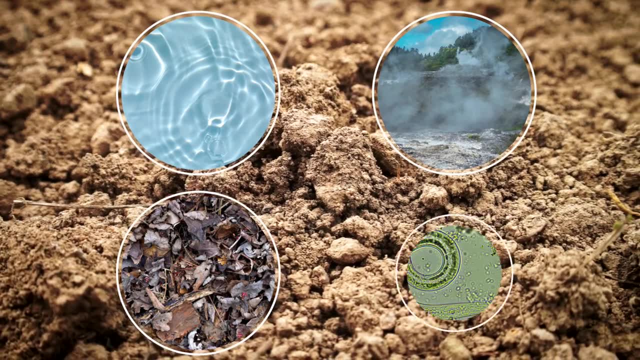 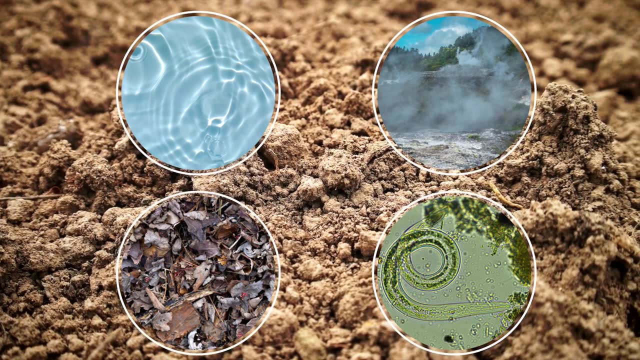 for plants and animals. Then these厊s of weathered rock mix with water gases from the atmosphere, decomposing organic matter and microorganisms to make soil. This mixture is what makes soil so unique and important. Without all of those peaces, it's just dirt. 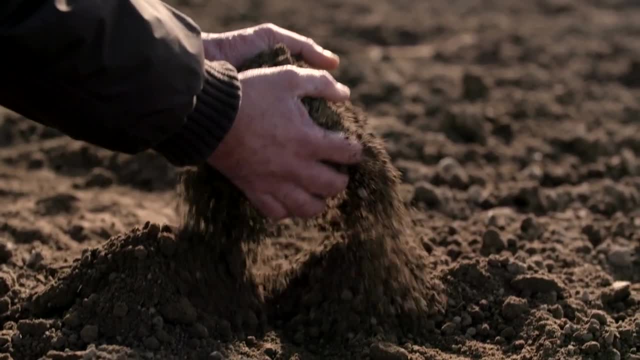 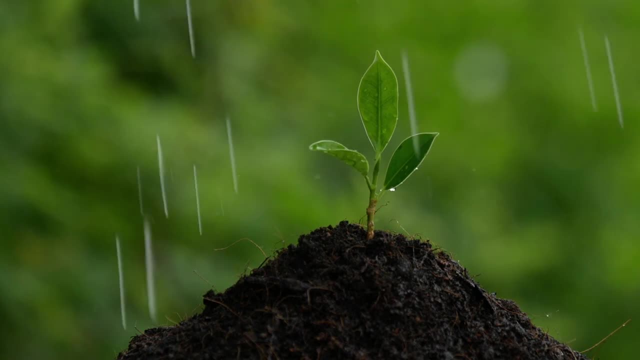 But weathering's role isn't over. when rock caves have to be persuaded to provide water to livelihood, rules snapping disappearרא. once rocks have become part of soil, The soil itself is continuously weathered too. This leads to erosion. when materials like rocks, minerals 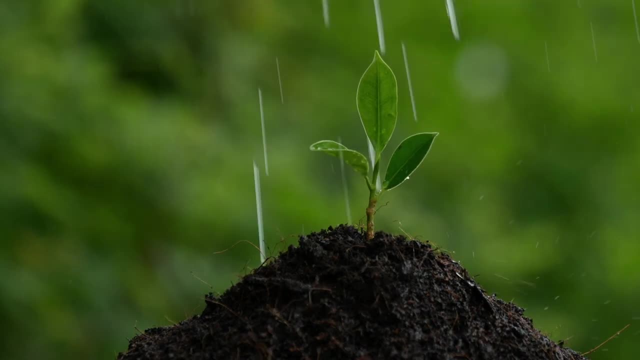 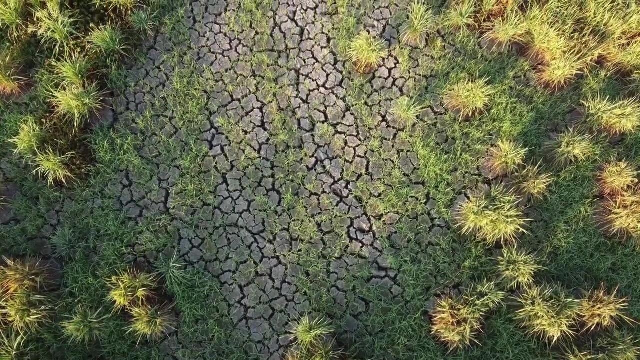 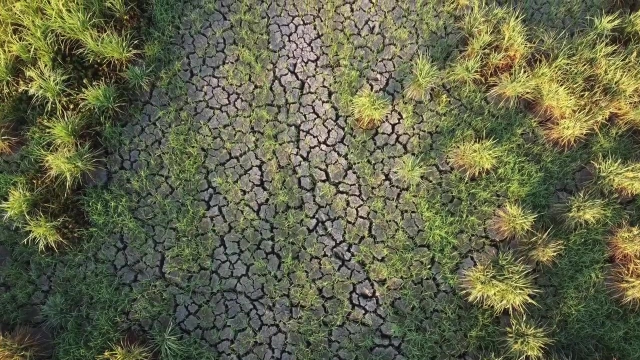 or the soil they're all mixed up in, are moved around by forces like wind and water. Unfortunately, the erosion of soil can cause lots of problems for the local environment. What kind of issues do you think can happen when soil is eroded? Pause the video here and write down your thoughts. 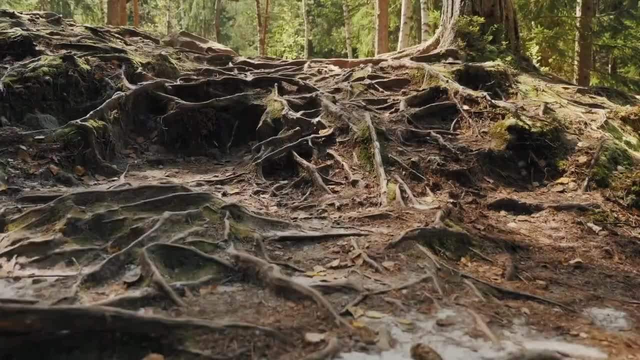 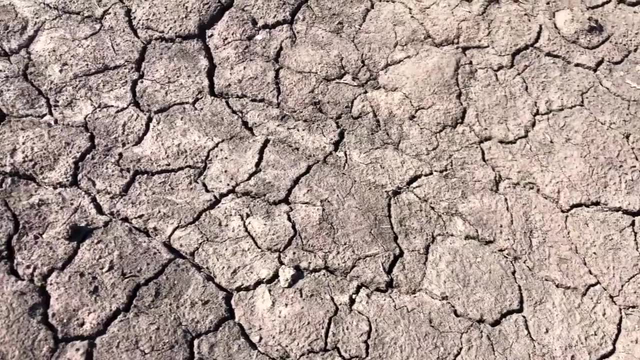 in your guided notes. Soil is essential to life on Earth. When it's eroded away, plants can't get the nutrients they need to grow, which means animals can't get the plants they need for food either, Without soil to hold them in place. rocks and dirt from deeper underground are often also eroded, which can clog up rivers with extra sediment. Plus, soil is very absorbent. Without this layer to soak up, all the rain areas start to flood more easily, which can cause a lot of problems for the environment.